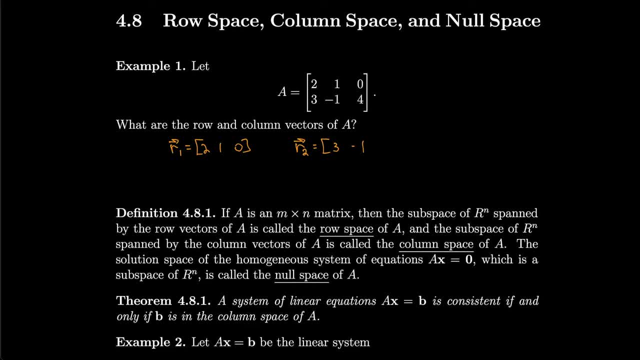 so 3, minus 1, 4.. As far as column vectors go, the first column vector is just the first, column 2, 3.. Second column vector is the second column, 1, minus 1, and the third column vector is the 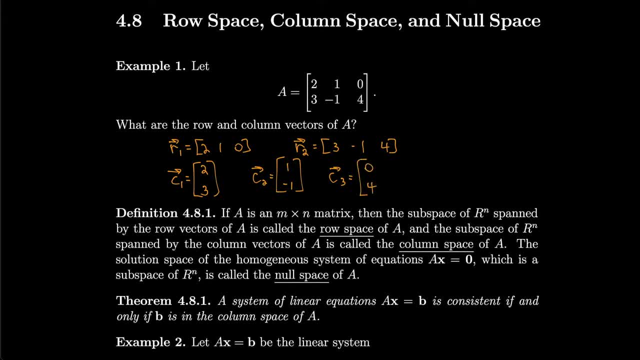 third column 0, 4.. If A is an educational video, please add punctuation in the appropriate places. If A is an M by N matrix, then the subspace of Rn spanned by the row vectors of A is called the row. 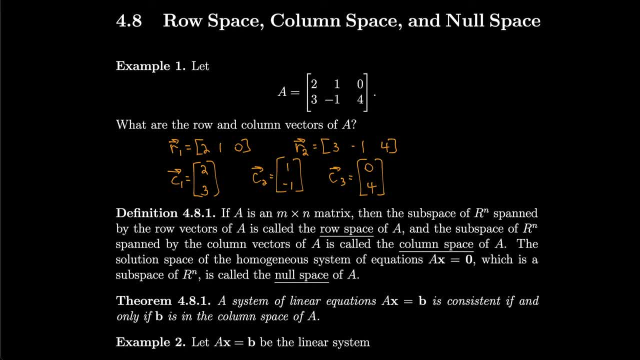 space of A and the subspace of Rn spanned by the column vectors of A is called the column space of A. The solution space of the homogeneous system of equations Ax equals 0, which is a subspace of Rn, is called the null space of A. So that's all the possible x's that make Ax equals 0,. 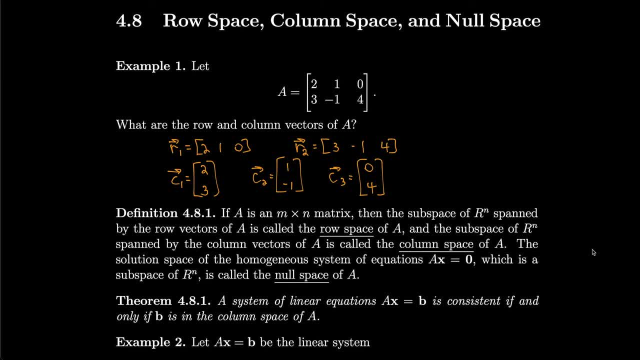 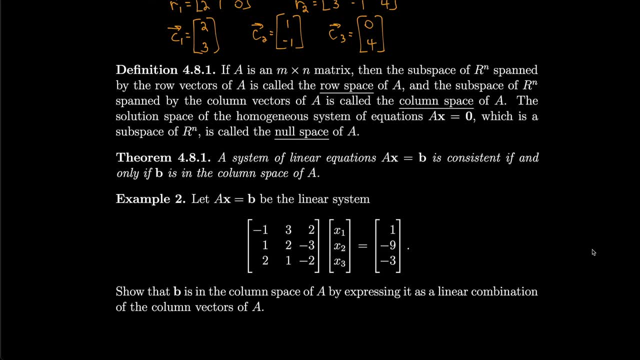 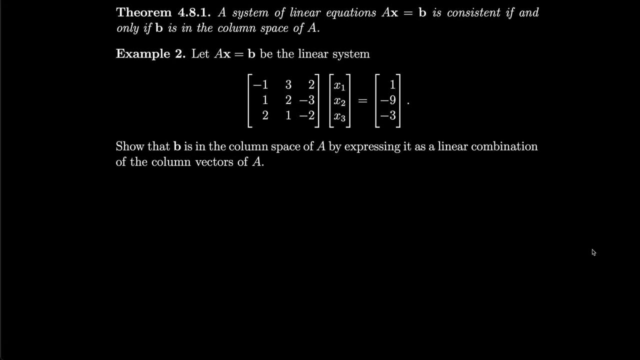 which is the column space of A. We call that the null space A system of linear equations. Ax equals b is consistent if, and only if, b is in the column space of A. So let's take advantage of that theorem. How about we let Ax equal b be the 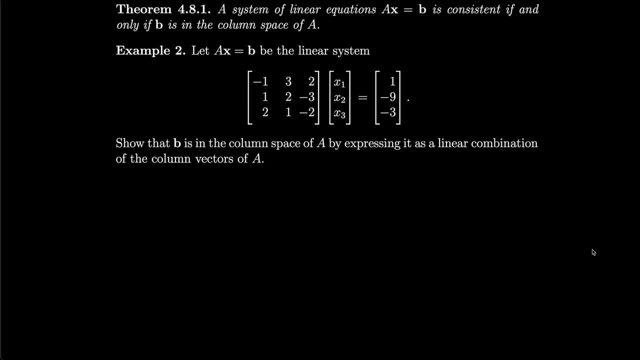 linear system given below. Let's show that b is in the column space of A by expressing it as a linear combination of the column vectors of A. So what we'll do is We'll try to take this matrix over here and put it in reduced row echelon form. So let's adjoin it to b. 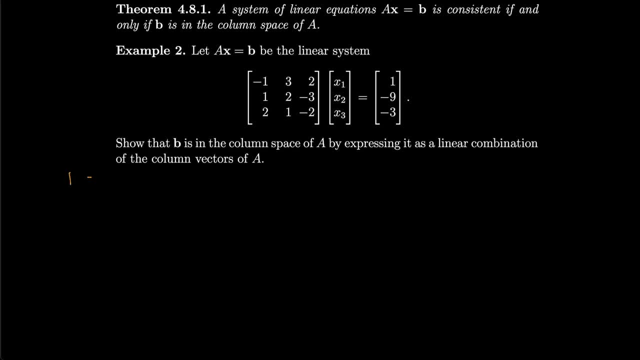 So I'll write 1 minus 3 minus 2 minus 1, because I'll multiply the top row by minus 1 in order to get a leading 1.. And then I will subtract it from this row to get a 0 and double it and subtract it from that row. 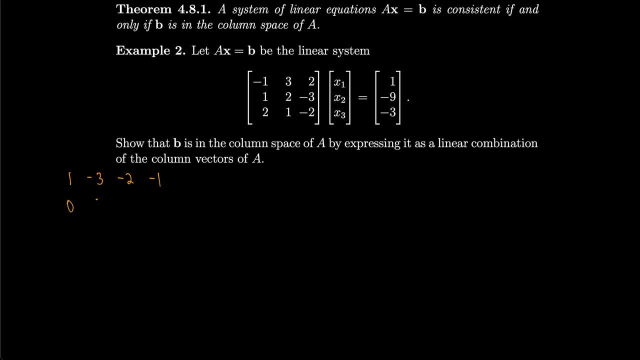 to get 0, so I'll get 0, 5, minus 1, minus 8, because the minus 9 will subtract off a 1 or subtract off a negative 1, so it'll add 1, get minus 8. and my last row: 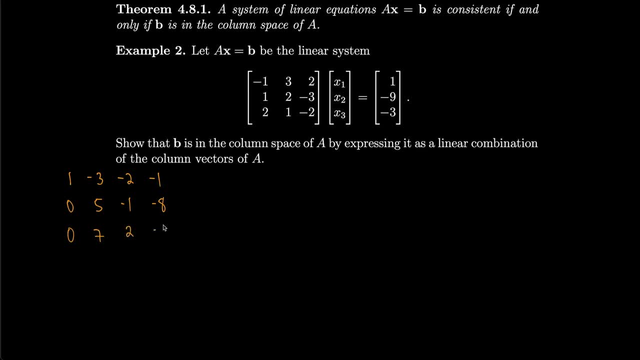 becomes 0, 7, 2, minus 1.. Okay, let's further reduce that. so I'll divide this by 5 so I can get a 1 over here, and I'll add multiples to get zeros over here, so I'll get 1, 0, minus 13 fifths. 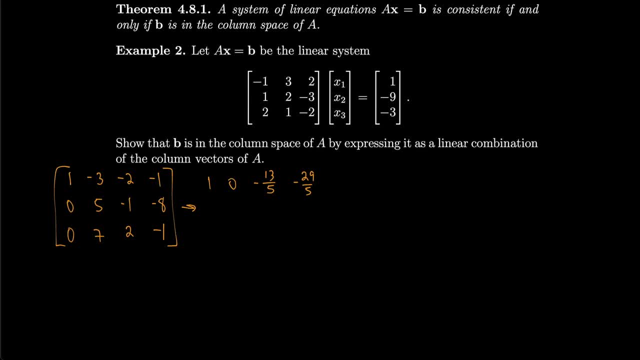 minus 29 fifths, 0, 1, minus 1 fifth minus 8 fifths and 0, 0, 17 fifths and 51 fifths. Okay, let's keep going, because we're almost there. The bottom row of 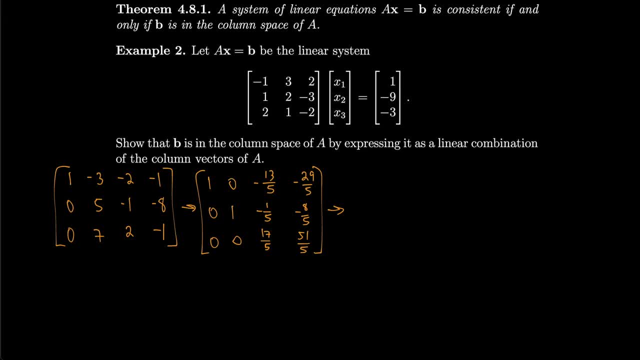 the row will divide by 17 fifths and I'll get a 1, and then I'll just add multiples of that to these rows to cancel out these, to get zeros. So I'll end up with 1, 0, 0, 2, 0, 1, 0, minus 1, and 0, 0, 1, 3.. So that means that I have x1. equals 0, 0, 2, minus 1, and 0, 0, 1, 3.. So that means that I have x1 equals 0, 0, 2, minus 1, and 0, 0, 1, 3.. So that means that I have x1 equals. 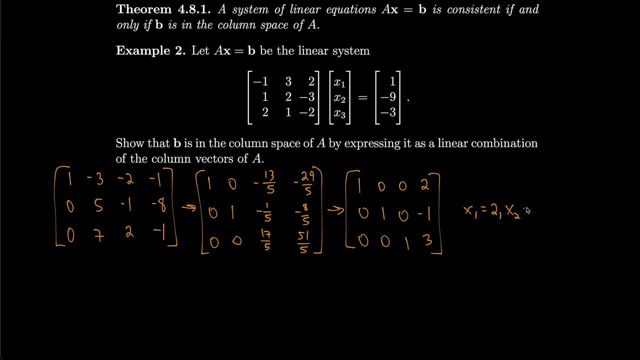 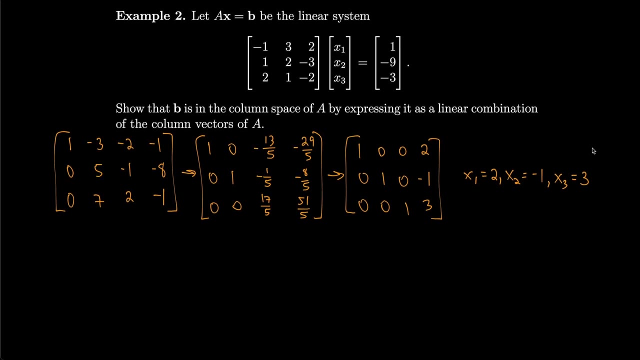 2, x2 equals minus 1, and x3 equals 3.. So let's see, I'm gonna take some linear combination of column vectors of A and try to get this B out of it. so let's write the column vector of A. 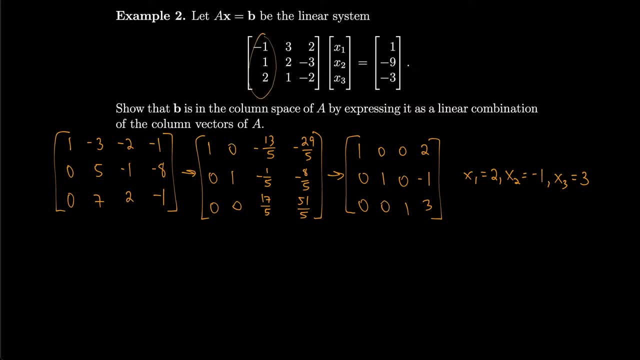 vectors of A. We've got that minus 1, 1, 2, and we've got 3, 2, 1, and we've got 2, minus 3, minus 2.. Those are column vectors. 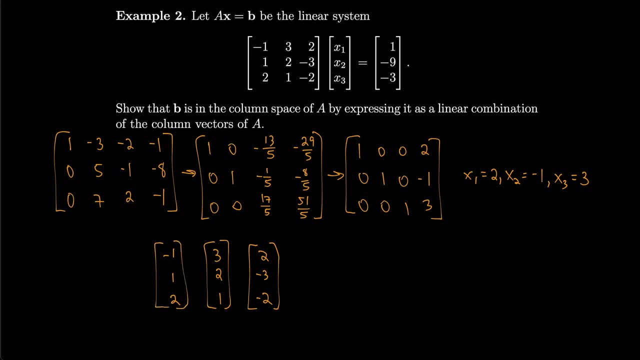 We want to take some suitable multiples of those to get to 1, minus 9, minus 3.. But notice, what we solved for over here are the x's that multiply by these column vectors to equal b. So these are precisely the coefficients that we need. So we'll just take two of this. 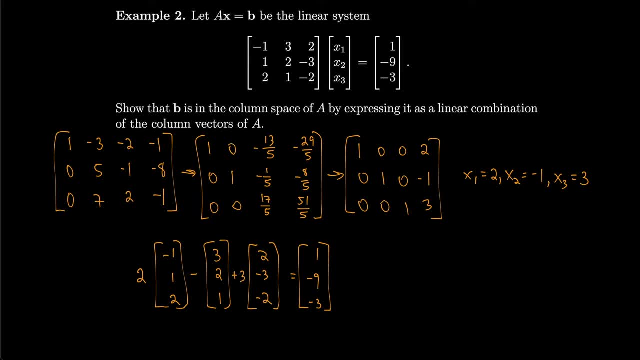 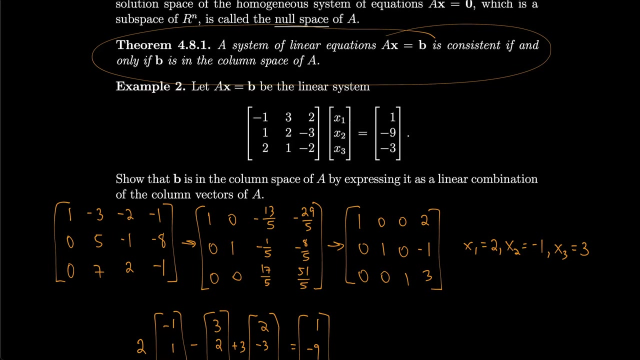 minus 1 of this, plus 3 of this, And notice that'll actually work, because minus 2,, minus 3,, plus 6, equals 1, and so on. So it kind of makes sense that a system of linear equations will be consistent if, and only if, b will be in the column space of A. 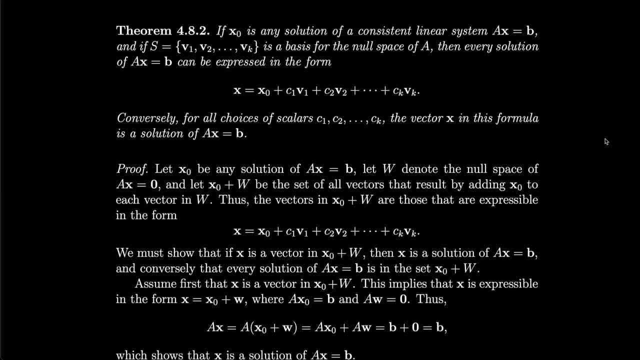 If x0 is any solution of a consistent linear system, A x equals b and if s equals v1 through vk is a basis for the null space of A, then every solution of A x equals b can be expressed in the form x equals x0 plus c1, v1 and so on, through ck, vk. Conversely for all choices of scalars c1. 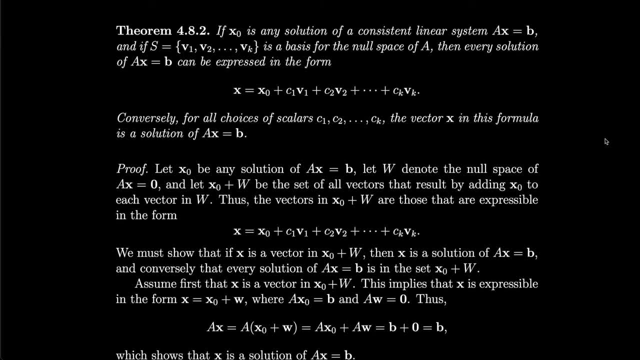 through ck. the vector x in this formula is a solution of A x equals b. So no matter what solution we have of the linear system A x equals b, if we take a basis for the null space, then we can write every possible solution in terms of that one solution we got. 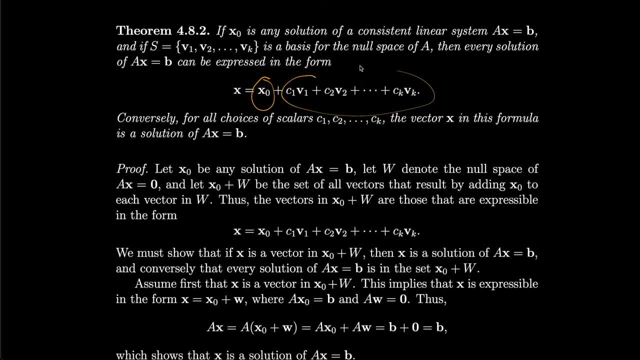 and some linear combination of the basis vectors To prove this. let x0 be any solution of A, x equals b. So let's take a null space of A, x equals 0 and let x0 plus w be the set of all vectors that result by adding x0 to each vector in w. 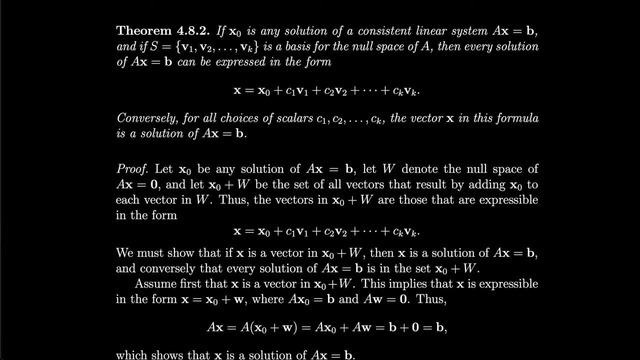 So then the vectors in x0 plus w are those that are expressible in the form: x equals x0 plus some linear combination of the basis vectors. We're just taking x0 and just adding it to vectors in w, and the vectors in w can be expressed in terms of basis vectors. 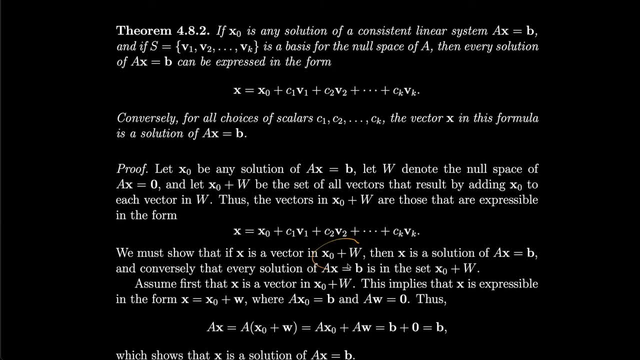 We have to show that if x is a vector in x0 plus w, then x is a solution of A, x equals b And conversely, that every solution of A, x equals b is in the set x0 plus w. So let's assume first that x is a vector in x0 plus w. 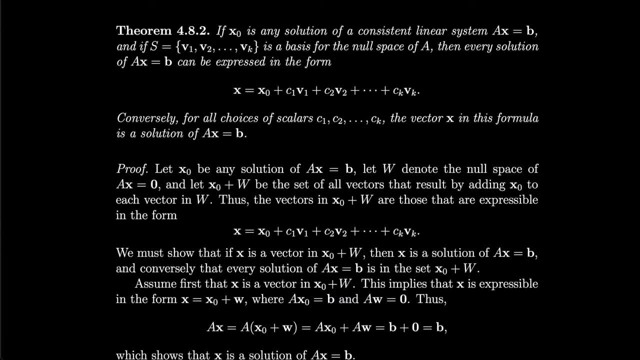 This implies that x is expressible in the form x equals x0 plus w, where A x equals 0 equals b and A w equals 0. We have to have that A x equals b and A w equals 0. Because that's what was our assumption to begin with. x0 was a solution of A x equals b. 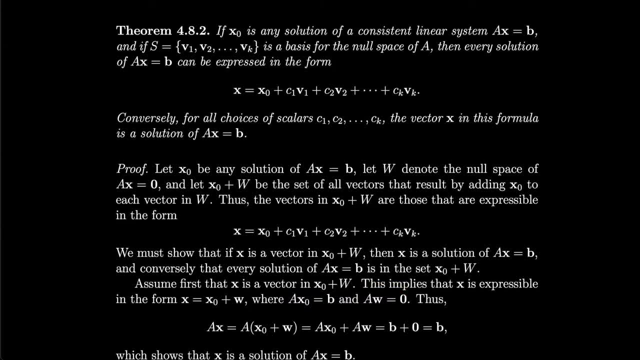 And we have to have A w equals 0. if we're looking at the null space, Remember, A x equals 0. And we're looking at some vector w in w. Okay, so then, if we look at A x equals A times x0 plus w. 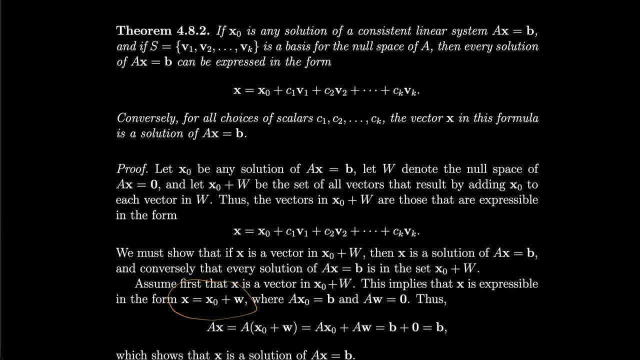 then because remember, it's got to be the form x equals x0 plus w, so we'll just replace x with x0 plus w. Then we can distribute the A. but we already know A x equals b, so I'll just replace A x0 with b. 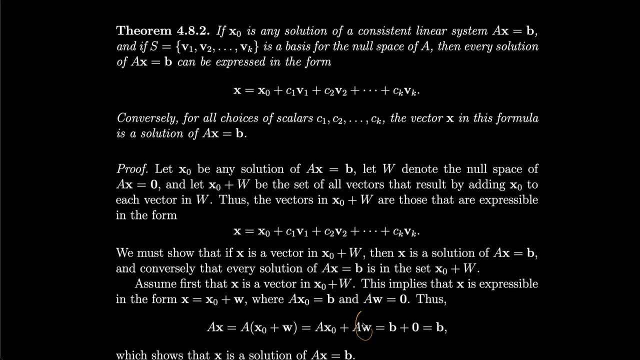 And we know A w is 0, so we'll replace A? w with 0.. So we get that we have b plus 0 equals b. but that means that the original A x we started with has to equal b. So that means that the x, which is equal to x0 plus w. 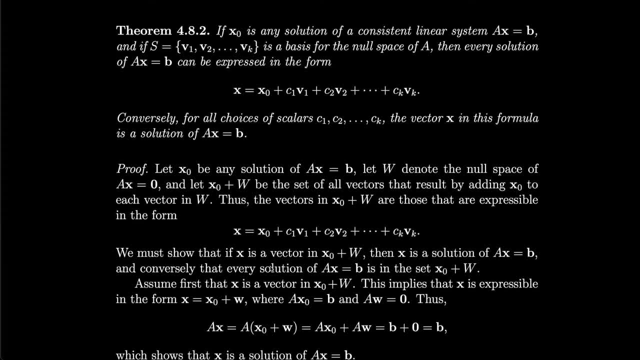 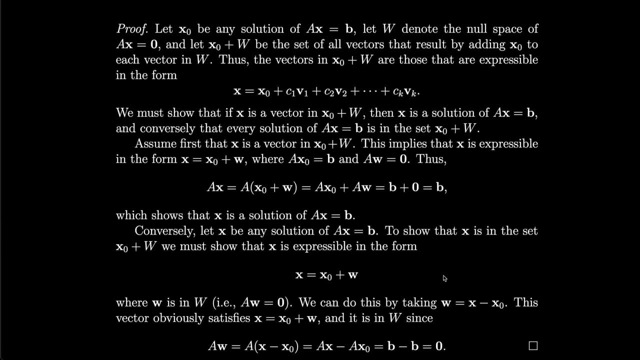 or x0 plus w, is in fact a solution of A. x equals b, So that gives us 1.. So that means that we have to show that x can be written as x0 plus w, where w is some vector in w the null space. 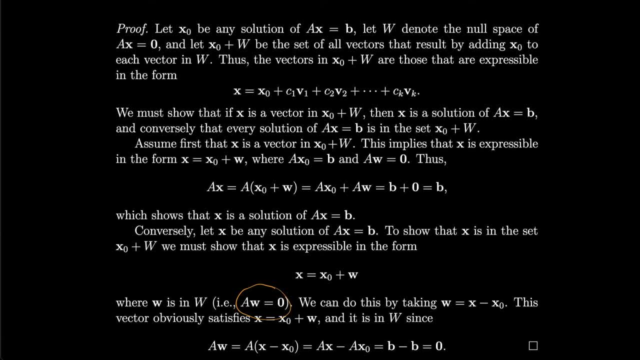 So that means that the same thing is saying that A times w is 0.. We can do this by taking w equals x minus x0.. That vector is a solution of A x equals b. So that means that we have to show that x is in the set x0 plus w. 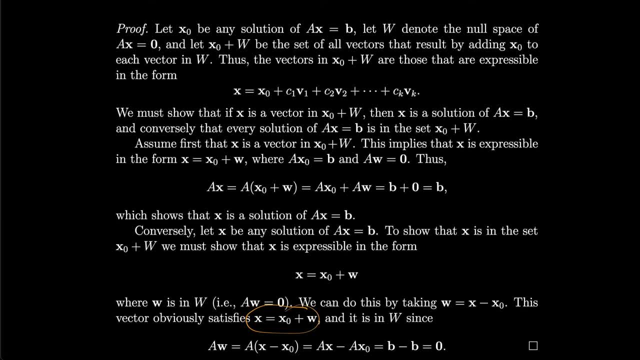 So that means that the vector will obviously satisfy: x equals x0 plus w. So now we just have to show it's in w. but it is because if we look at A times w, then that's A times x minus x0, because that's what we set w to be. 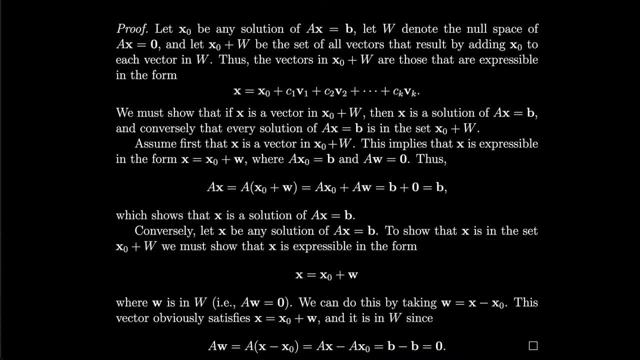 Again, distribute the A, We get A x and A x0.. But A x is equal to b. A x0 is also equal to b. So we get that. But b minus b is 0, gives A w equals 0.. 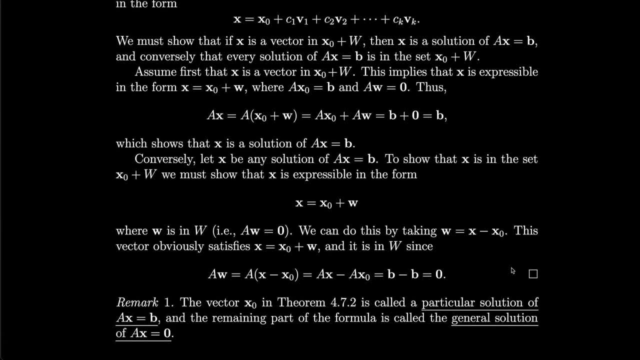 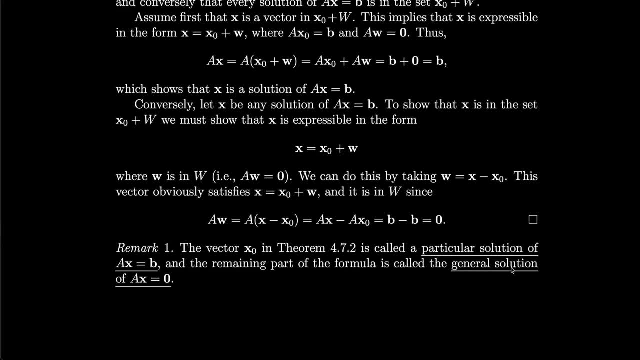 So that means w is in fact in the null space. So that gives us both directions of this proof. The vector x0 in this theorem is called a particular solution of A x equals b. The remaining part of the formula is called the general solution of A x equals 0.. 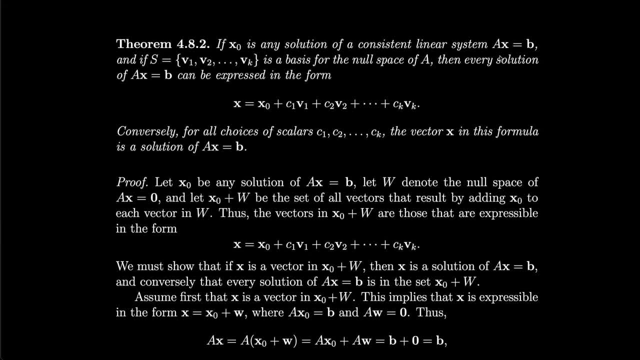 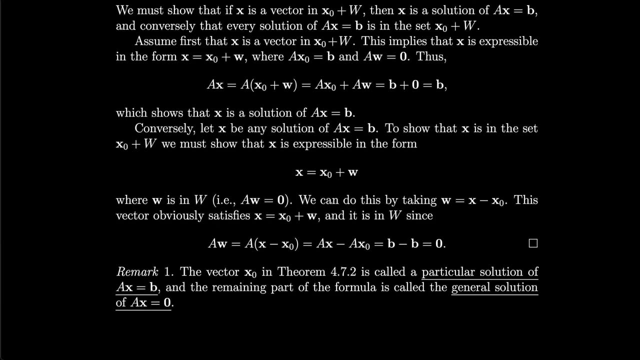 So essentially, what this theorem is saying is that if we have a particular solution and we have a linear constant and we have a combination of a general solution of the homogeneous equation- because that's what we're saying- the second part is that's a general solution of A. x equals 0,. 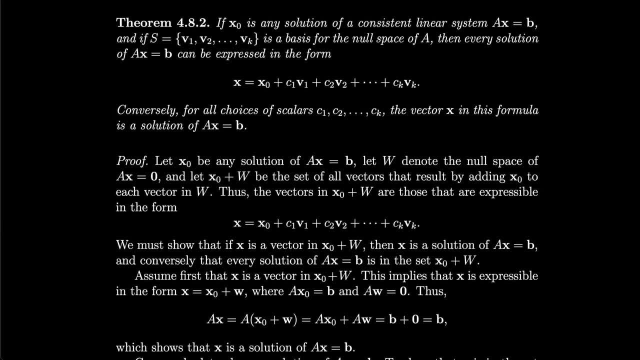 then that gives us the general solution of A: x equals b. We take a particular solution, we add it to a general solution of the homogeneous equation where instead of b we do 0, and we can get the general solution of A: x equals b. 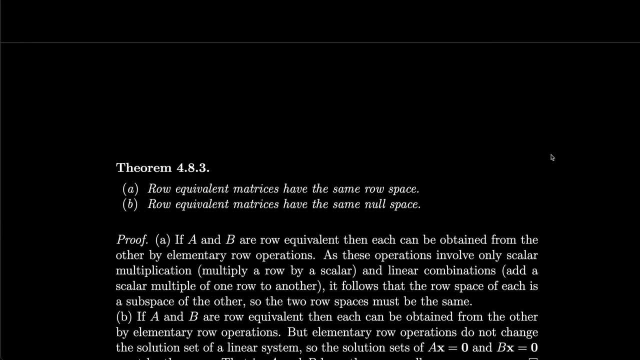 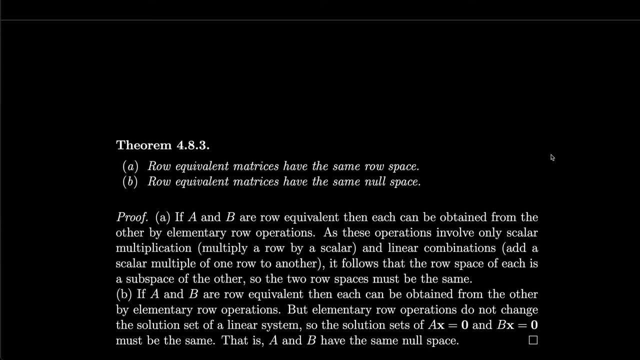 For our next theorem. we have that row-equivalent matrices have the same row space and row-equivalent matrices have the same null space. Notice, however, we specifically do not talk about the column space, because it's not true that row-equivalent matrices have the same column space. 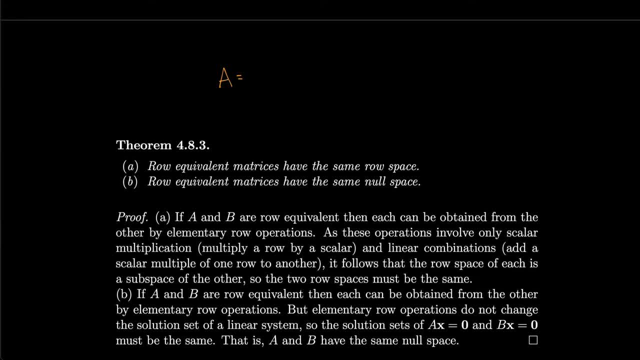 In other words, if I have some matrix, let's say A and let's write it as. let's say 1, 3,, 2,, 6,, for example. then notice that the column space, well, the first column- is 1, 2,. 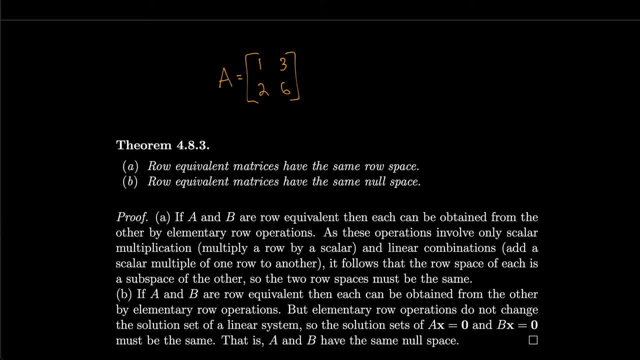 the second column is 3 times that. so you can see that the column space is just going to be has basis 1, 2.. You can build up both columns from that from the linear combination, If I do some elementary row operations. 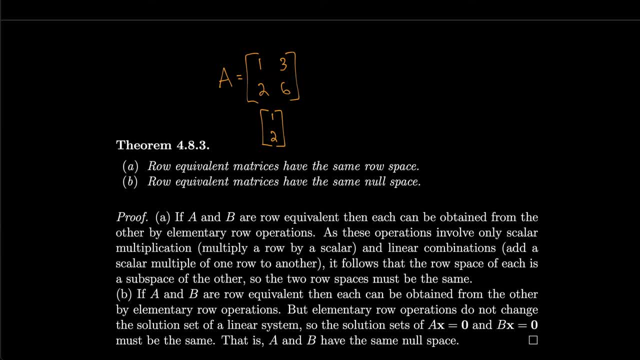 let's say I take 2 times the first row and I subtract it from the second, so then I would get b equals 1, 3, 0, 0,. new matrix: I made out of A by just taking the first row. 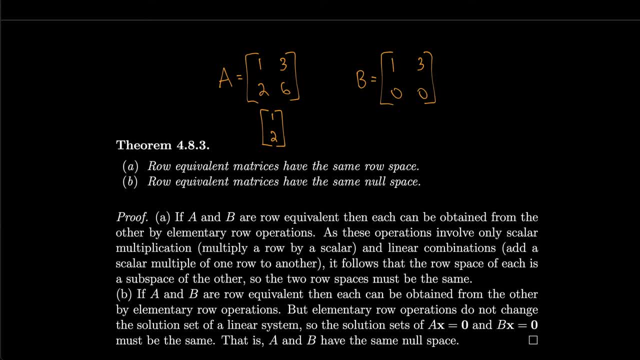 and subtracting twice that from the second row. so that's just an elementary row operation. I now have a column of 1, 0 and a column of 3, 0, so the second column is 3 times the first one. 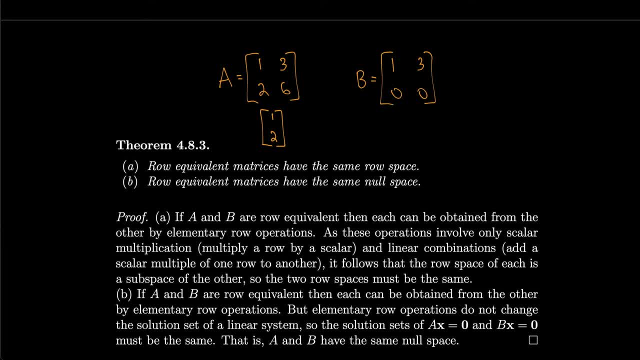 so that means that the basis for the column space of B is 1, 0.. And notice that these vectors are linearly independent. They do not form the same basis. This is not a multiple of this one, so they do not have the same column space. 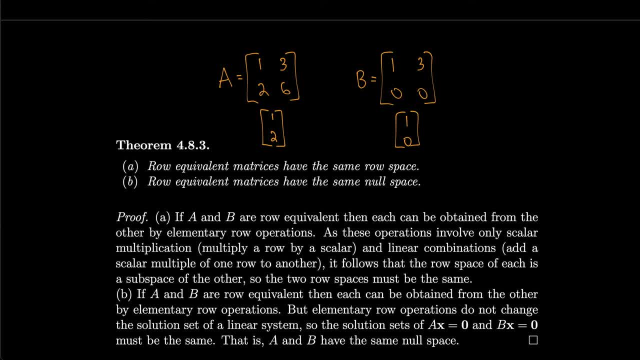 However, by this theorem, these matrices, because I only modified them by doing an elementary row operation, they do in fact have the same row space and the same null space, as we're about to prove. If A and B are row equivalent, then each can be obtained from the other by elementary row operations. 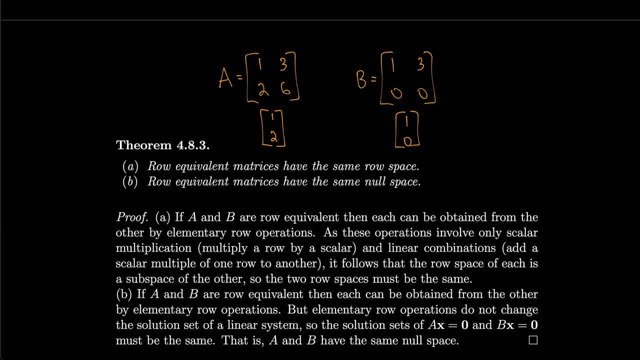 As these operations involve only scalar multiplication, say multiplying a row by a scalar and linear combinations, adding a scalar multiple of one row to another, it follows that the row space of each is a subspace of the other, so the two row spaces must be the same. 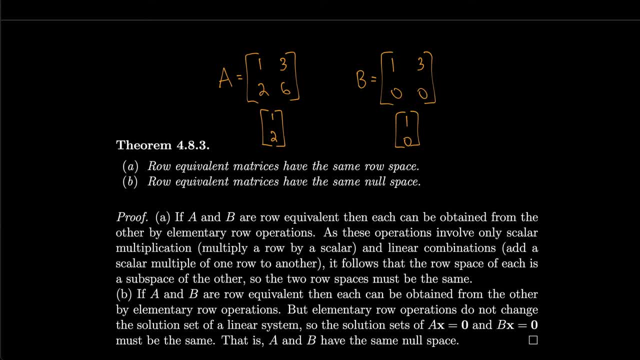 We're building up the row space through the linear combinations, essentially of the different rows. So when we do elementary row operations, all we're doing is new linear combinations. so it makes sense. it's not going to change the basis. Let's talk about the null space now, though. 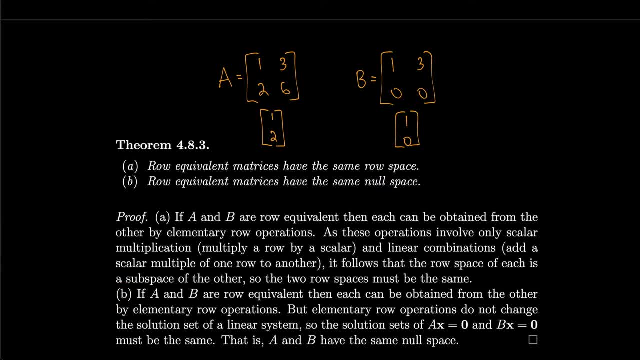 For part B of this theorem. if A and B are row equivalent, then each can be obtained from the other by elementary row operations. but elementary row operations do not change the solution set of linear system. That's the whole. point is that we can keep doing elementary row operations. 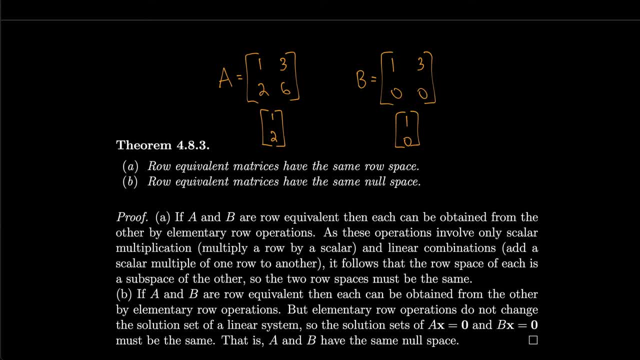 to get into reduced row echelon form and then we know what the solution is. So that means that the solution sets of A x equals 0 and B x equals 0, if we change from A to B for the elementary row operations. 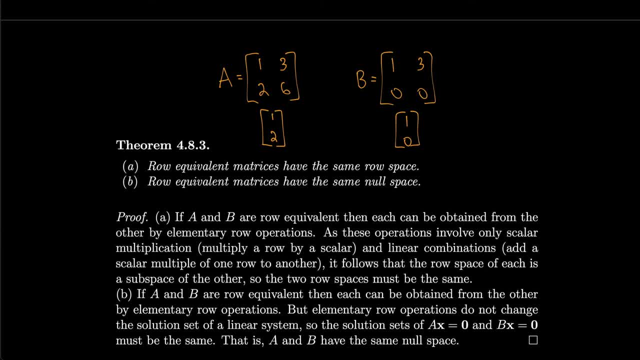 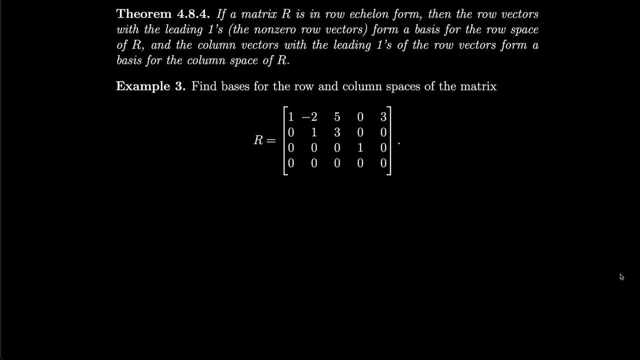 they must be the same, so that means that they must have the same null space. If A matrix R is in row echelon form, then the row vectors with the leading ones, the non-zero row vectors, form a basis for the row space of R. 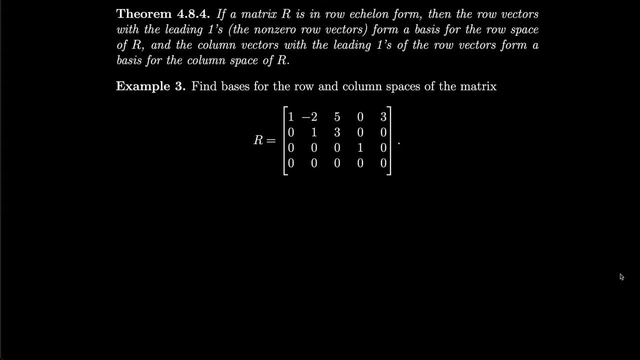 and the column vectors, with the leading ones of the row vectors, form a basis for the column space of R. Let's find bases for the row and column spaces of the matrix R given in this example. So all we have to do is write out the rows that have a leading one. 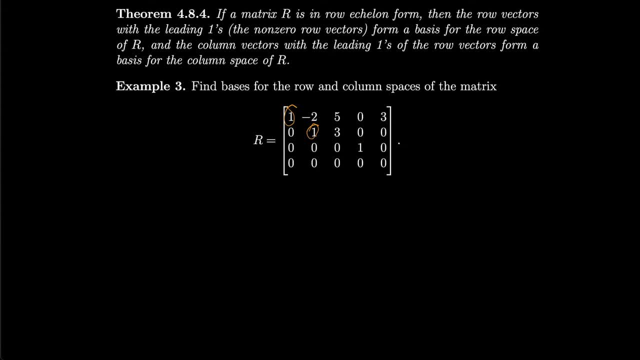 So here's one, here's one, here's one. The last one has no leading one, so we will omit it. So, row one, column vector: the row vector is one minus two, five, zero, three. The row two vector is zero one, three, zero, zero. 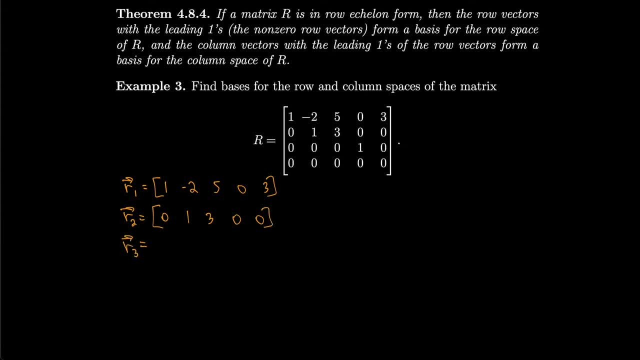 The row three vector is zero, zero, zero, one, zero, And that's a basis for the row space of R. Now for the column space. We need the columns that have leading ones. So let's see, We've got this. one has a leading one. 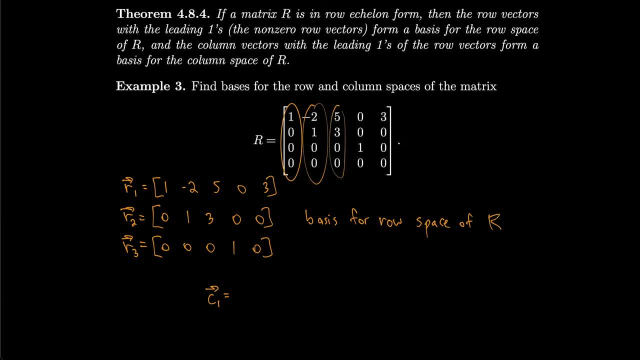 this one and we'll skip this one because there's no leading one. So this one. So there's only three, even though there's five columns. So we'll have: C1 is one zero zero zero. C2 is minus two: one zero zero. 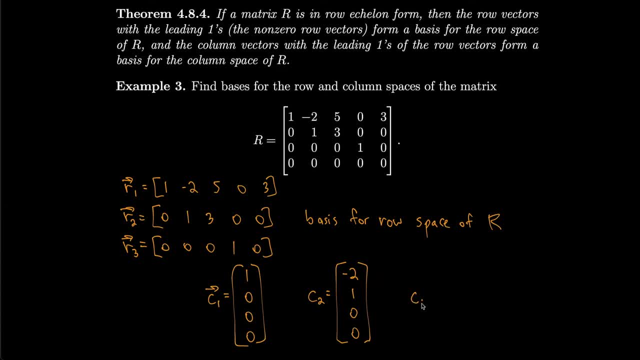 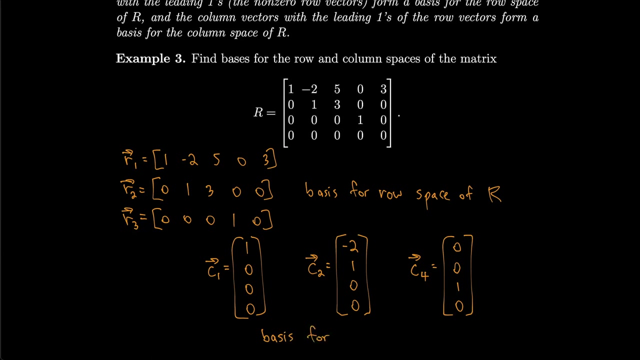 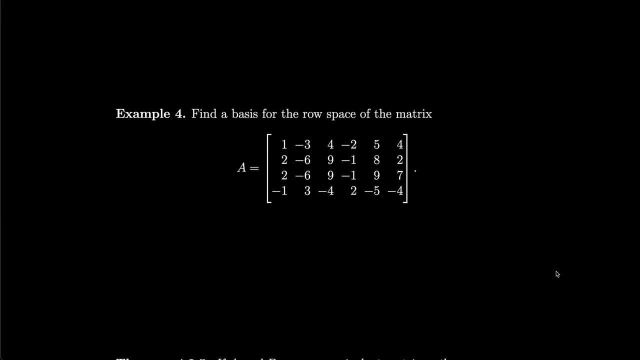 And our last column vector. for the basis I'm going to say it's C4, because I skipped C3.. So C4 is zero, zero, zero, zero And that's a basis for the column space of R. How about we next find a basis for the row space? 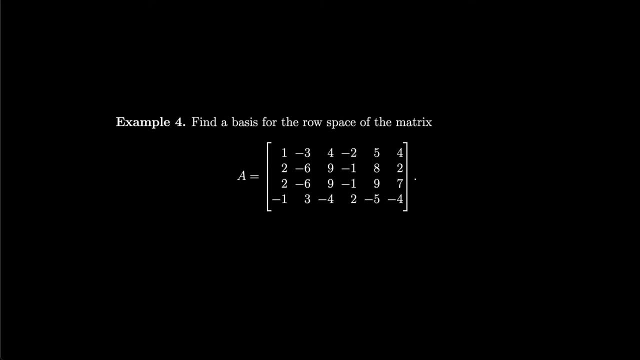 of this matrix A. Well, the first thing we have to do is put A into row echelon form. We don't have to reduce it, So we'll write the row echelon form for A. I'm not actually going to go through all the steps. 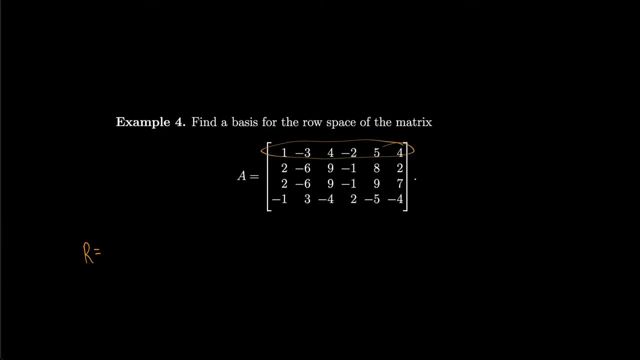 but basically you'll take some multiples of the first row and add them to the other rows, So that way you can get zeros underneath that. You'll get a leading one over there. All these will be in a row. All these will end up being zero. 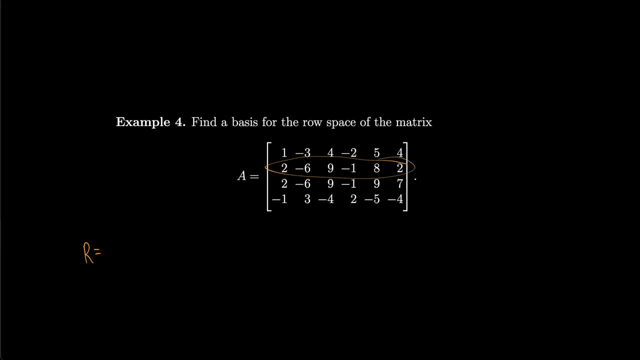 And then you'll get a leading one over here. by dividing and so on, You should end up with a row echelon form of one minus three, four minus two, five four, zero, zero. one three minus two minus six. 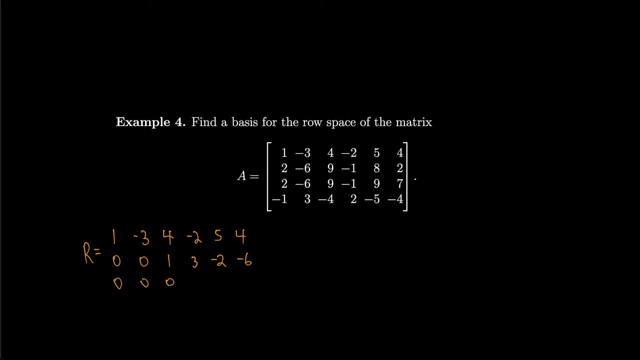 Zero, zero, zero, Zero, one, five, And the last row is just all zeros. Okay, so now it's pretty easy to see that the basis for the row space is just these row vectors that have leading ones in them. not the last row, because it just has zeros. 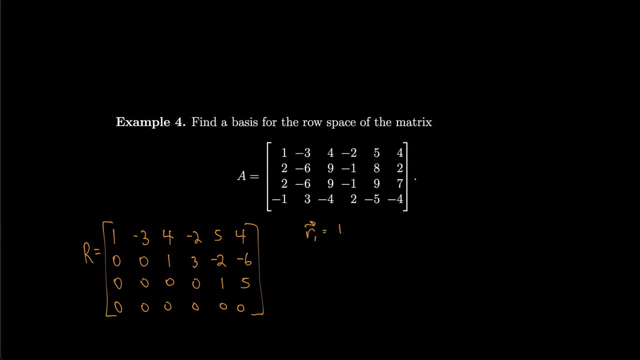 So that's row one, which is one Minus three, four minus two, five four. Row two, that's just zero, zero, one, three minus two minus six, And row three, which is zero, zero, zero, zero, one five. 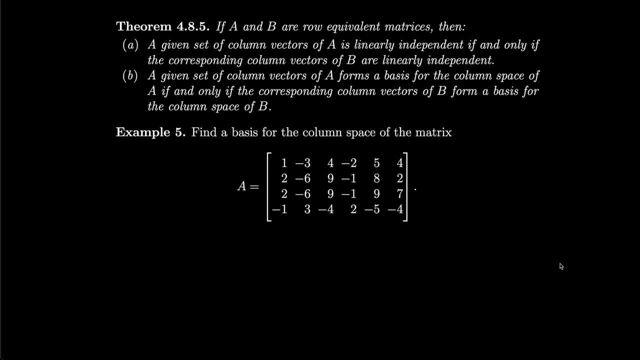 If A and B are row-equivalent matrices, then a given set of column vectors of A is linearly independent if, and only if, the corresponding column vectors of B are linearly independent And a given set of column vectors of A forms a basis for the column space of A. 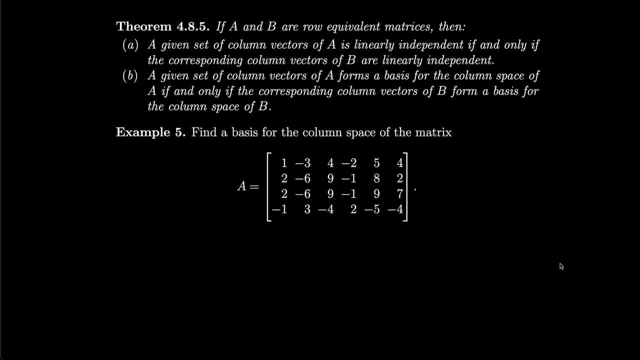 if, and only if, the corresponding column vectors of B form a basis for the column space of A. So what we're doing is we're trying to come up with a good way of finding a basis for the column space of a matrix, but also be able to reduce the matrix. 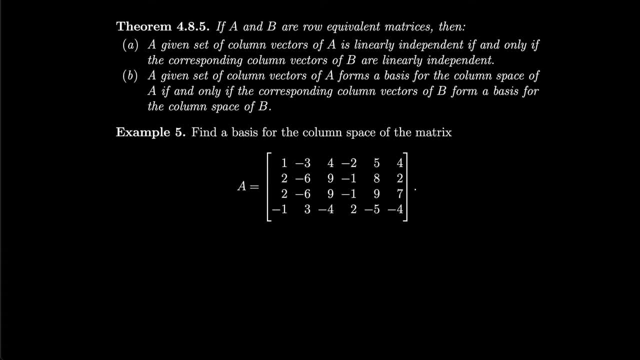 Because, remember, it's not going to have the same column space as the reduced matrix. If we use elementary row operations, it'll change the column space potentially. So we have to work a little more carefully. What we'll do is we'll take A and we'll reduce it the same way as we did in the last example. 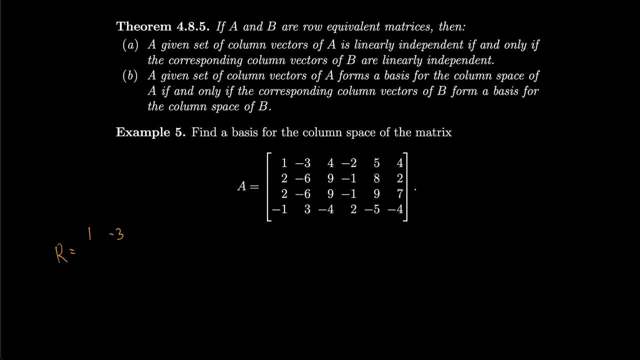 So we'll get one minus three, four minus two, five, four, zero, zero. one three minus two minus six, zero, zero, zero, zero, one, five and zero, zero, zero, zero, zero. 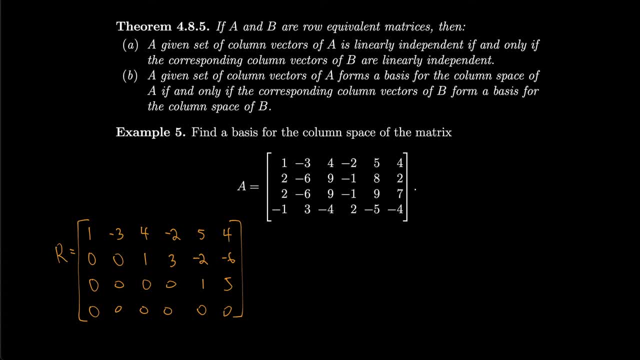 So that's my row echelon form for A. So now I can get a basis for the column space of my row echelon form. That'll just be the C1, that first one, But I'm going to use C's for my original matrix A. 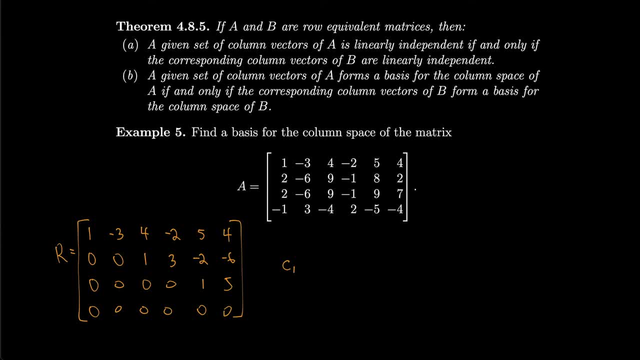 So I'll call the columns for R primes. So I'll say: C1 prime is the first column vector for R. So that's just one zero, zero, zero. Remember I'm only looking for column vectors that have leading ones in them. 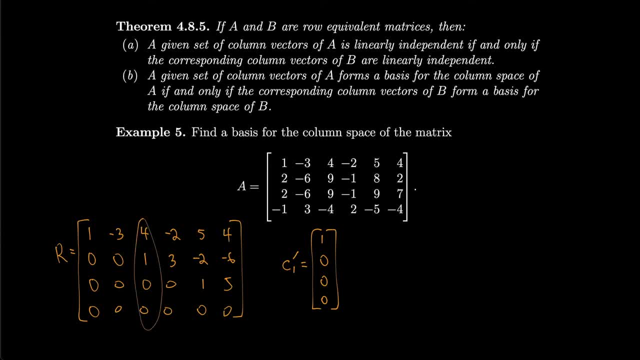 There is no leading one in that second one, so I'm going to skip it and go to column three. So that's my second basis vector. So that's four. one zero, zero And then C5 prime, because, remember, I'm skipping. 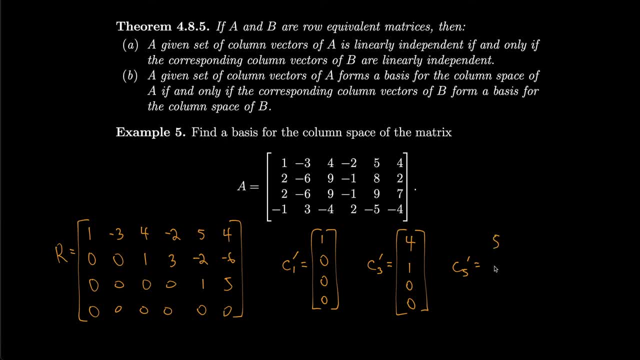 there's no leading one over, there will just be five minus two, one zero, And that is a basis for the column space of my row echelon form R. So I need to be able to get to a basis for the column space of my original matrix. 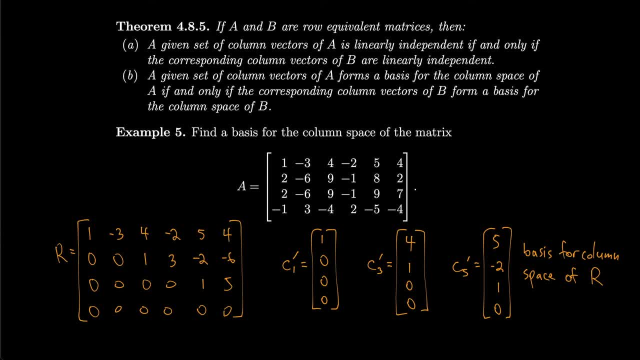 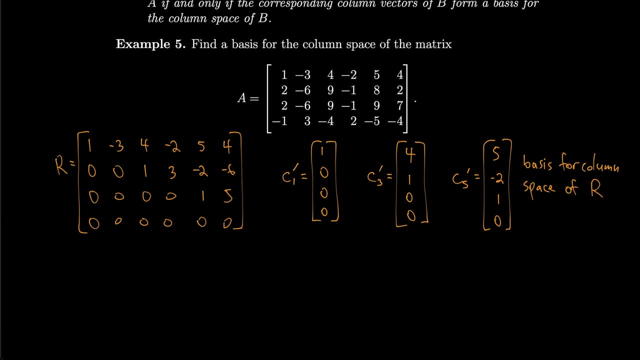 This theorem says that the column vectors correspond, So that means that the basis for the column space of A is just going to be formed of C1, C3, and C5, where those are my original column vectors. So I'll look at C1. 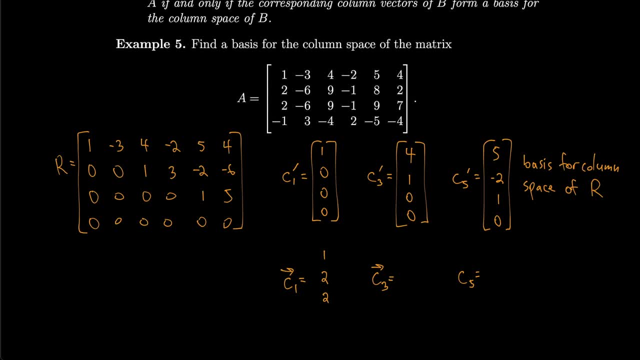 So that must be one, two, two minus one. And then, because I skipped two in my row echelon form, I'll skip two in my original matrix and I'll go straight to column three. So that's four, nine nine minus four. 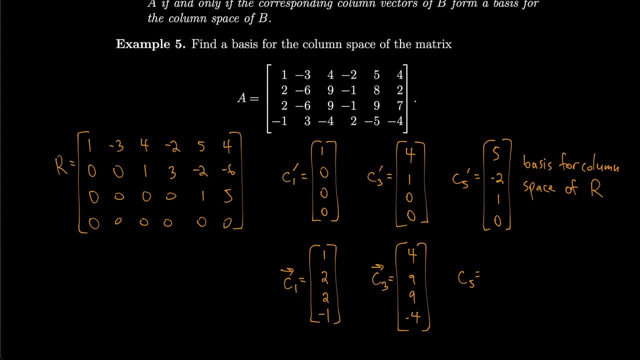 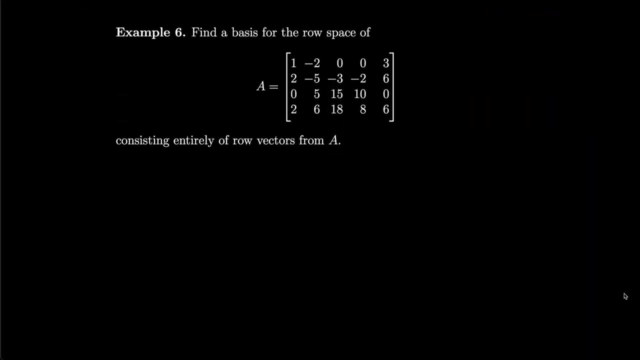 And for C5, I'll get five, eight, nine minus five And that'll be a basis for the column space of A. So notice, it is different than ours, but it is still possible to find out what it is based on ours. 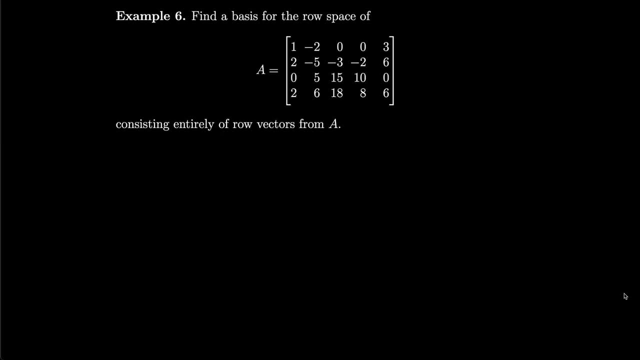 Let's next find a basis for the row space of A consisting entirely of row vectors from A, So we could put this in row echelon form and then figure out a basis for A, just like we did in example four. However, if we do that, 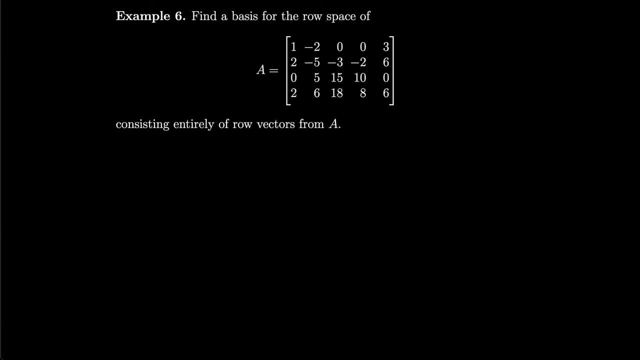 it will not consist entirely of row vectors of A. That basis will have different vectors in it that aren't the vectors of A. So it would be nice if we could use that theorem. we just did, but that only applies to column vectors and we're trying to do this. 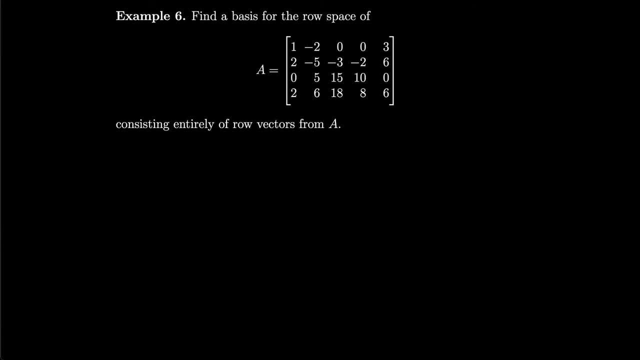 for the row space with row vectors. So what we could do is we could transpose A so that the row vectors become column vectors and then use that theorem. So how about we do that? We'll write A transpose, as let's see, the first row becomes the first column. 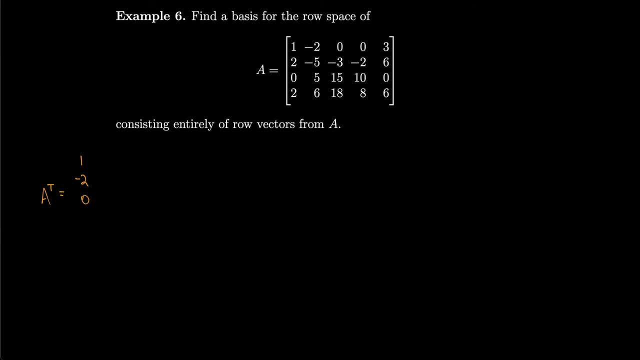 so that's one minus two, zero, zero, three. then second row, second column, so two minus five minus three minus two, six and then zero, five, fifteen, ten, zero and two, six, eighteen, eight and six. 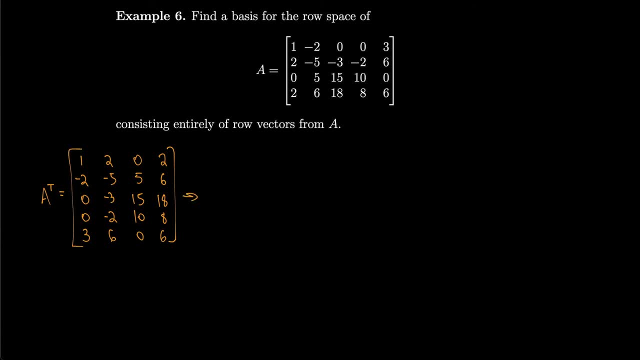 Okay, so now we'll reduce that. If I put this in row echelon form, it's a little bit of work, so I'm going to skip some of those steps, but it becomes one, two zero, two zero one. 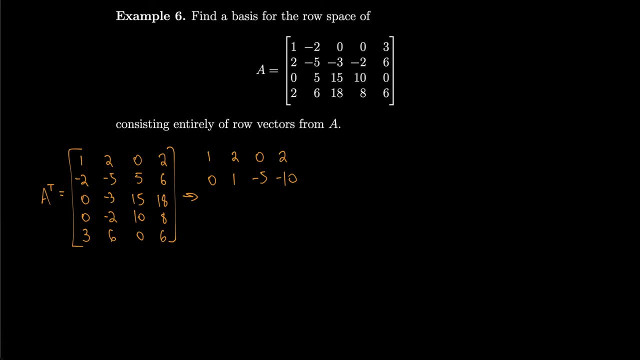 minus five minus ten, zero, zero, zero. one, zero, zero, zero, zero and zero, zero, zero zero. Okay so now I can write off the vectors that form the column space for A transpose. Let's see for C1,. 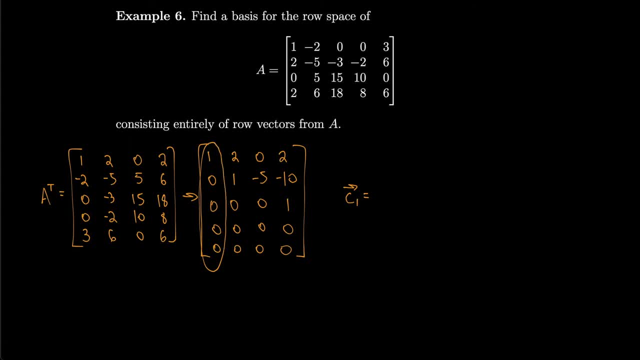 right, that'll be the vector, the column vector that corresponds to the first one in my row, echelon form, because it has a leading one in it. So I'll read that off as one minus two, zero zero three. I'm not even going to bother writing. 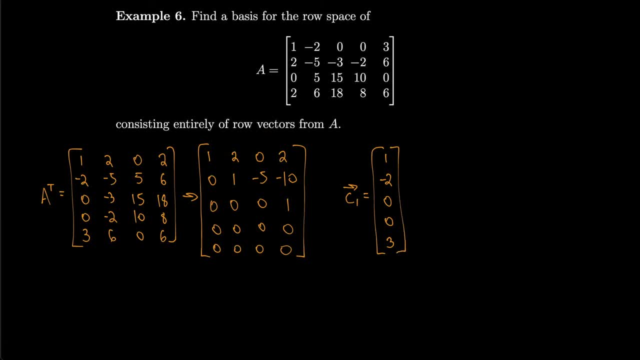 the basis for my row echelon form, because I don't need it. I'm just going to go straight to the basis for A transpose, for the column space of A transpose. So there's a leading one in my row echelon form. so that means that 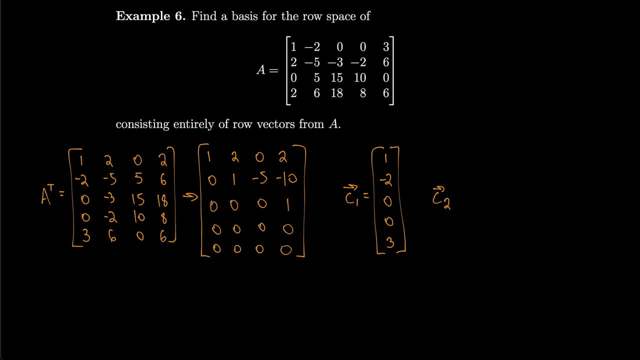 the second vector will work in my basis. So that's two minus five minus three minus two six, And now I just need: oh well, there's no leading one over there, so I'll skip that. Leading one over there means: 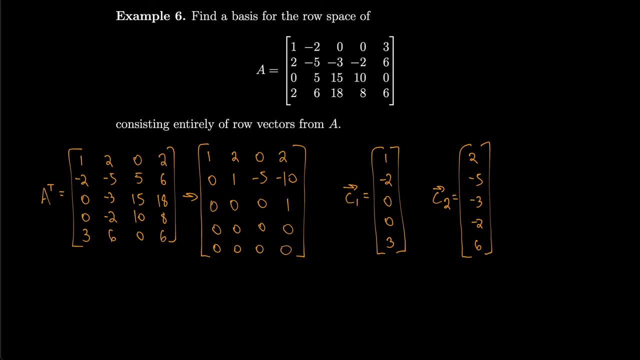 that. I look at the last column for A transpose, so that's C4.. So that's two six eighteen eight six, Okay. so that's a basis for the column space of A transpose. So to get back to A, 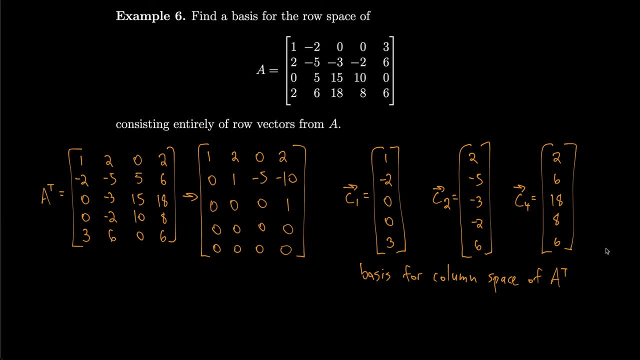 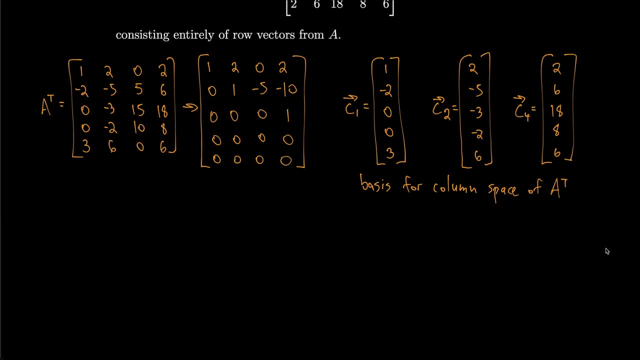 all I have to do is transpose again, because transpose and A transpose will flip my columns back to rows, So that means that my first column becomes my first row, So I'll get row. one is one minus two zero zero three. 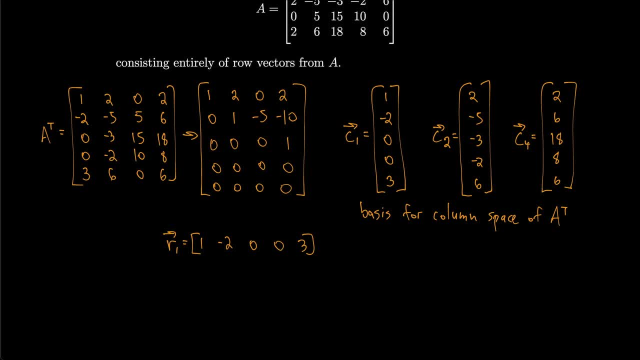 as it was before. I'll get my second column, my second row, so that's two minus five minus three minus two six, and I'll skip row three because I skipped column three, and I'll get. row four is two. 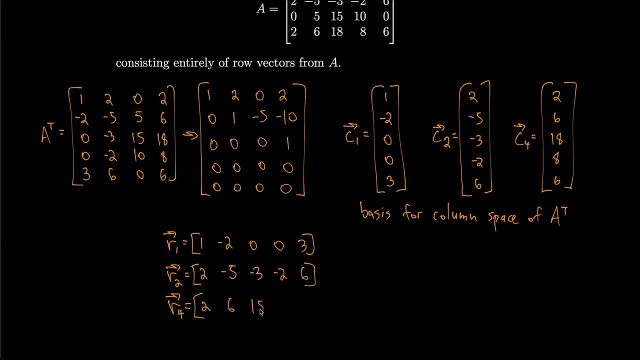 six, eighteen, eight and six, And that's a basis for the row space of A that's actually built up out of the rows of A. We could have found a different basis for the row space of A by putting A in row echelon form. 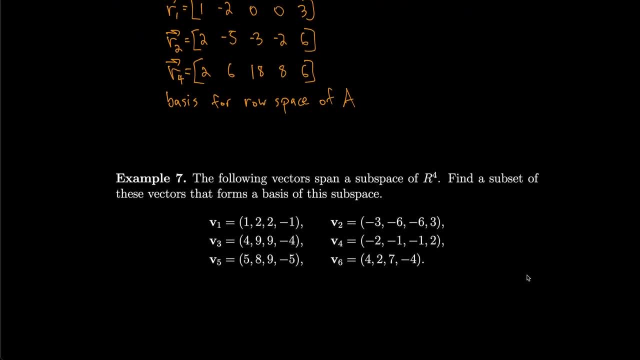 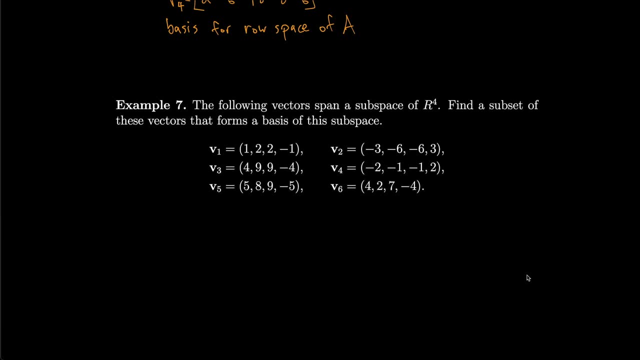 but that wasn't what the question asked for. in this space, The following vectors span a subspace of R4.. Let's find a subset of these vectors that form a basis of this subspace. Okay, so how about we write each of these vectors? 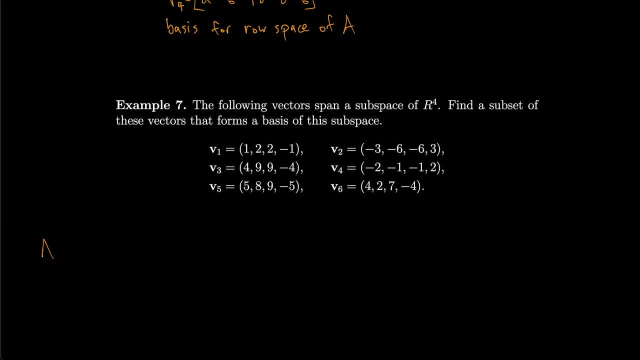 as column vectors in a new matrix- Let's call that matrix A. We'll write the first column vector as V1, so that'll be one, two, two minus one. then V2 will be minus three minus six, minus six. 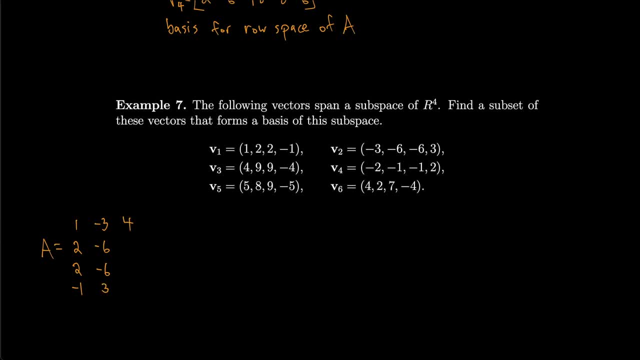 three, and we'll keep going like that. So four, nine, nine minus four minus two minus one minus one. two, five, eight nine minus five and four, two, seven minus four. And notice this is: 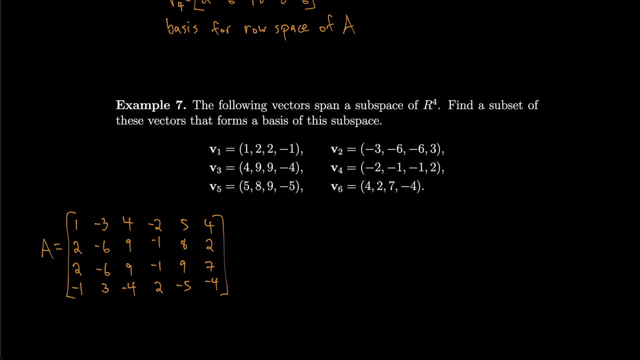 the same matrix that we already identified: the column space of. Remember that they're saying that these vectors span a subspace of R4, so the span of these vectors: V1,, V2,, V3,, V4,, V5, and V6. 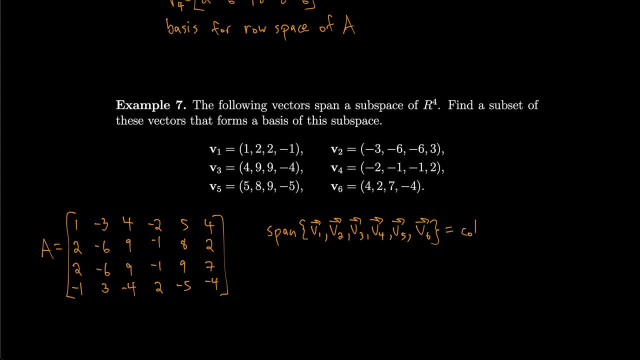 span the column space of A, So they form the column space. So if I just remove a couple of the extra vectors, a couple of the vectors that are linearly dependent on each other, then we can reduce this spanning set to a basis. 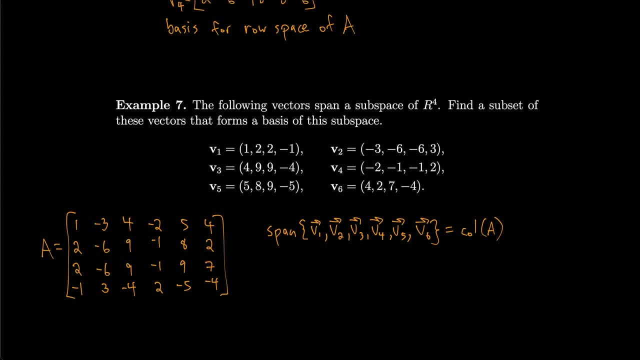 Because if the set spans and is linearly independent, it's a basis. So the fact that it spans and is not currently a basis implies we have some redundant vectors, which we know we do, because when we last looked at this matrix, we saw that the basis for 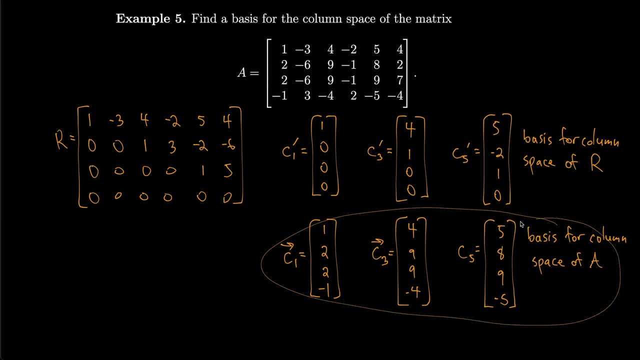 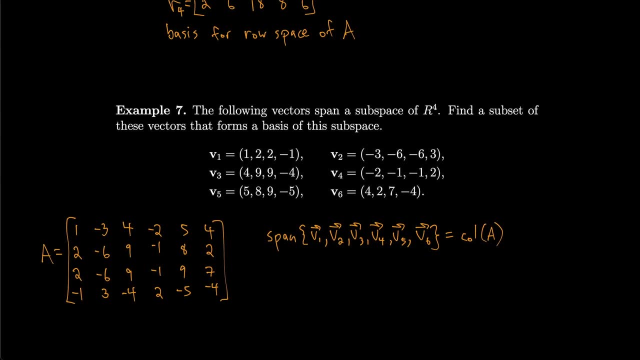 the column space was spanned just by C1,, C3, and C5. So that means that that's all we have to look at over here. We just need C1, C3, and C5. In that case, that's just. 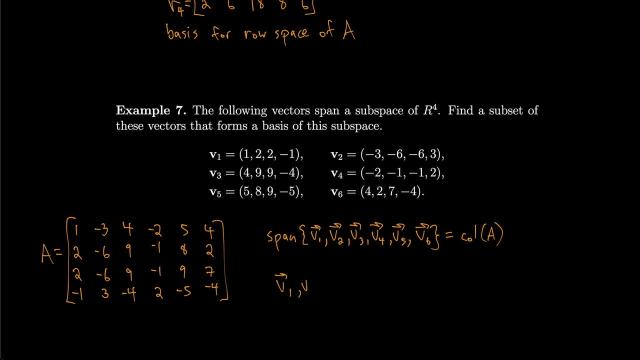 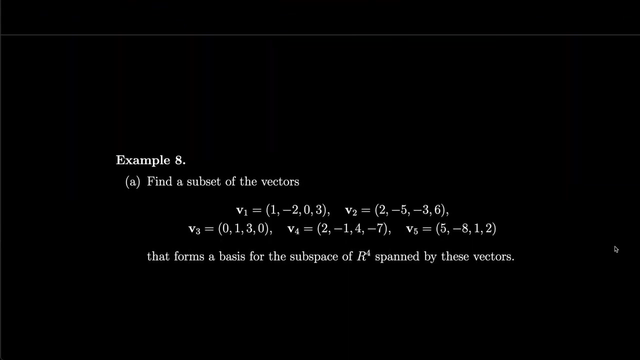 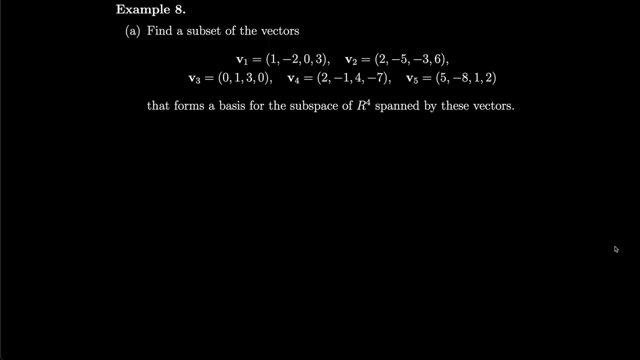 V1,, V3, and V5.. So that's what forms a basis for the span of V1, V2, V3,, V4,, V5, and V6.. How about we next find a subset of the vectors V1 through V5. 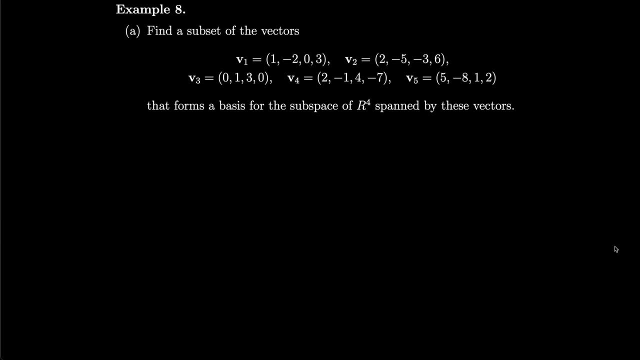 that forms a basis for the subspace of R4 spanned by these vectors. So again, I'll write them as the column vectors of a matrix. So I'll write 1, minus 2,, 0, 3 for V1.. 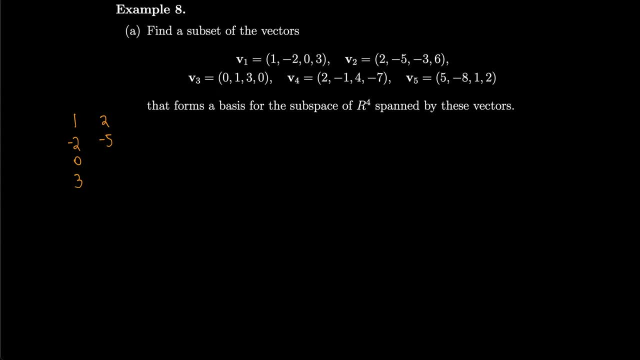 We'll write 2, minus 5, minus 3, 6.. So this one's V1, V2, and then 0, 1, 3, 0 for V3,: 2, minus 1,. 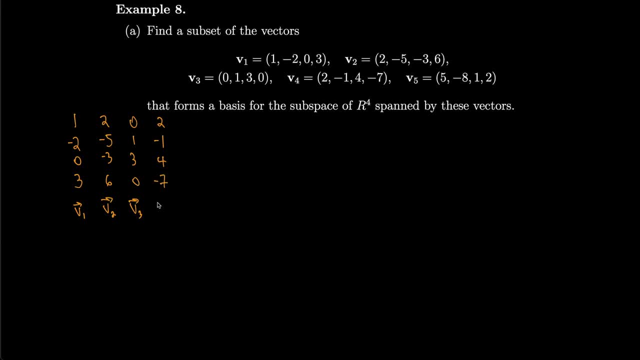 4, minus 7 for V4, and 5, minus 8, 1, 2 for V5.. Okay, so then I'll reduce this to get, let's say, 0s underneath over here, and by doing that, 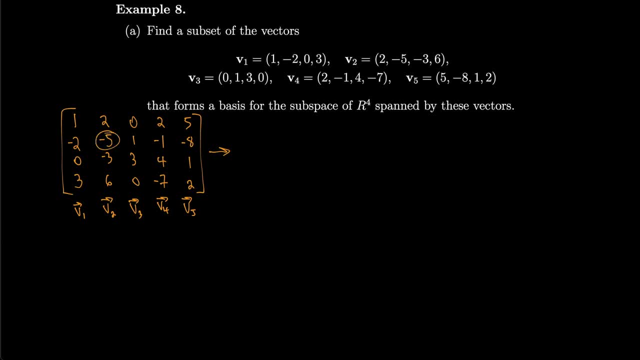 it looks like I can get a 1 over here. Just have to multiply the second row by negative 1.. So it looks like I can get 1, 2,, 0, 2, 5, then 0, 1,. 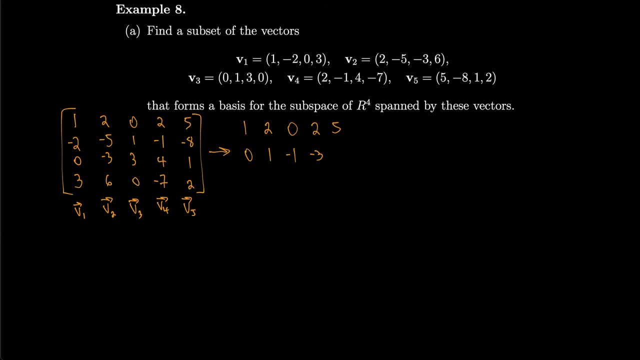 minus 1, minus 3, minus 2, and my third row I'll leave as 0, minus 3, 3,, 4, 1, and my last row: just subtract 3 at the first and get 0, 0, 0,. 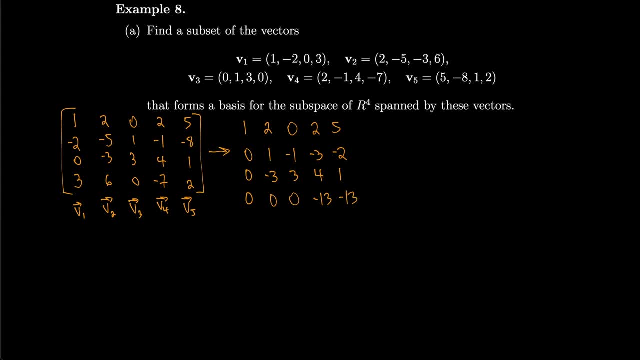 minus 13,. minus 13.. Okay, let's keep going. So further reduce it by getting a 0, 0, 0 over here and over here, So I'll get 1, 0,, 2,, 8,, 9,. 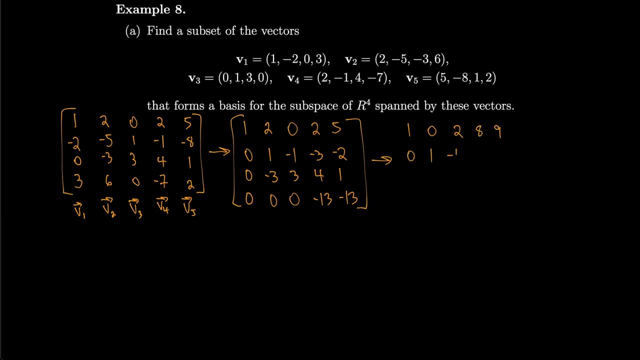 0, 1, minus 1, minus 3, minus 2, 0, 0, 0, minus 5, minus 5, and 0, 0, 0, 1, 1.. 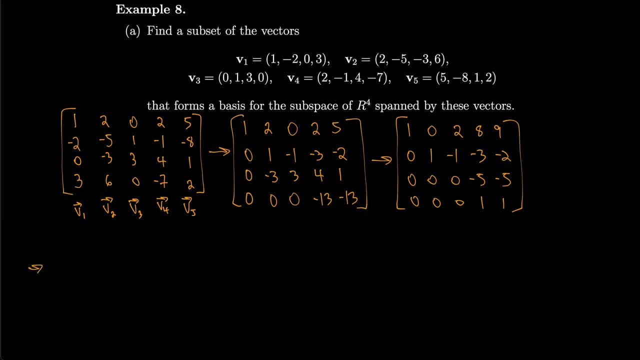 Okay, almost done. the this row and this row looks like i can cancel one of them out. i'll just take the last row, move it to the third row and then add five of it to the third row to make the that row zero. so on top. 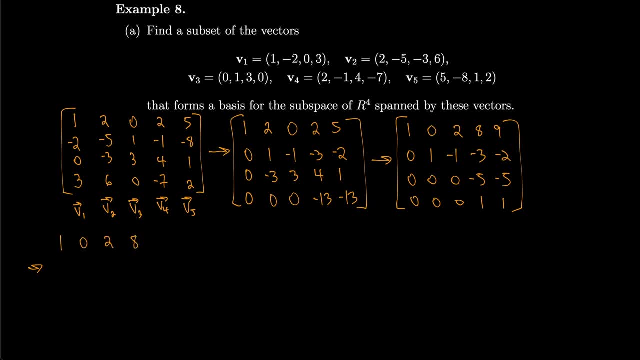 i'll get one zero two, eight, nine again. i'll get zero, one minus one, minus three, minus two again, but then my third row will be zero, zero, zero, one, one from the fourth row, and my new fourth row will just be all zeros. okay, so now uh. 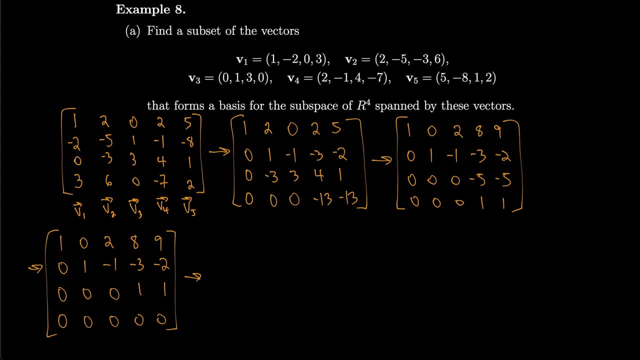 for pretty much done. i can just get zeros above this leading one by writing one zero two zero one and zero, one minus one, zero one, zero, zero, zero, one, one and zero, zero, zero, zero, zero. okay, so then i'm going to call these new vectors w1, w2, w3, w4 and w5. those are my new column vectors. notice that i have leading ones over. 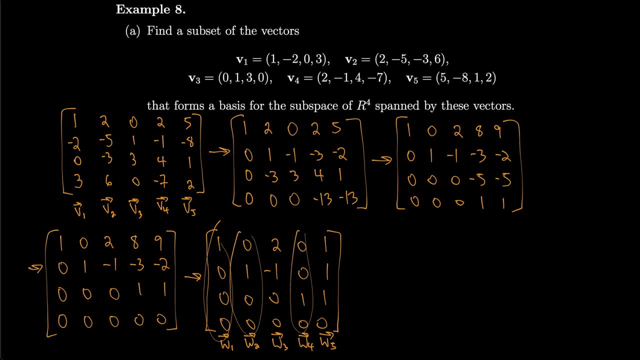 here, over here and over here at one, two and four. so that means that w1, w2 and w4 is a basis for the span of w1, w2, w3, w4, w5, just like the way that we figured out a basis for the span in the previous example. 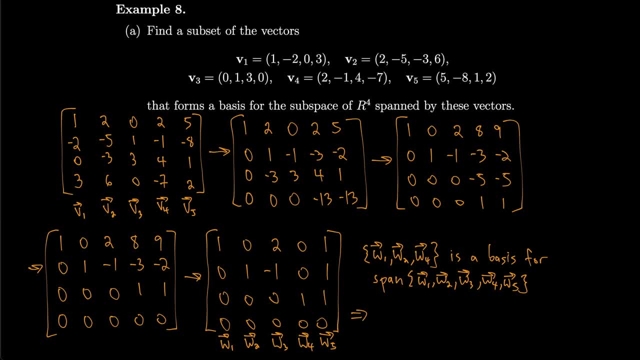 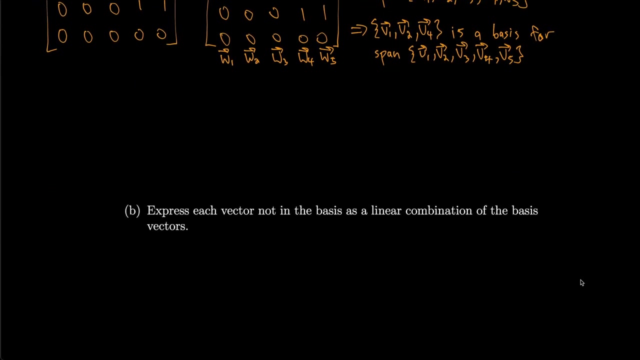 so that implies that w1- w1- we'll be a basis for the span of w1, w2, v3, w4 and V5.. Let's express each vector not in the basis as a linear combination of the basis vectors. Okay, so we skipped W3 and we skipped W5,. 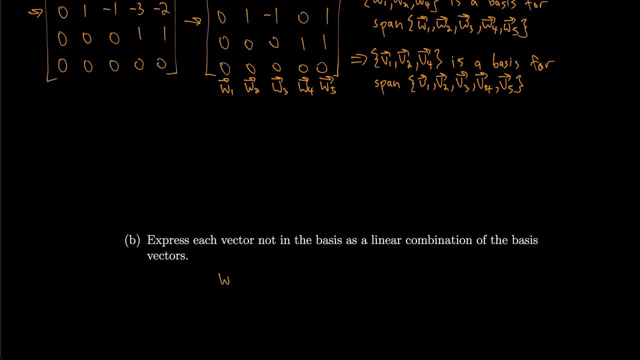 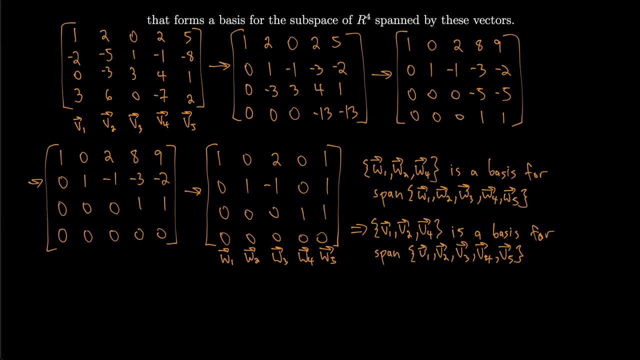 so those are the two we have to worry about. So let's write W3 as a linear combination of the other vectors in the basis, other column vectors and W5.. So let's see W3,. well, W3, it looks like we could just take. 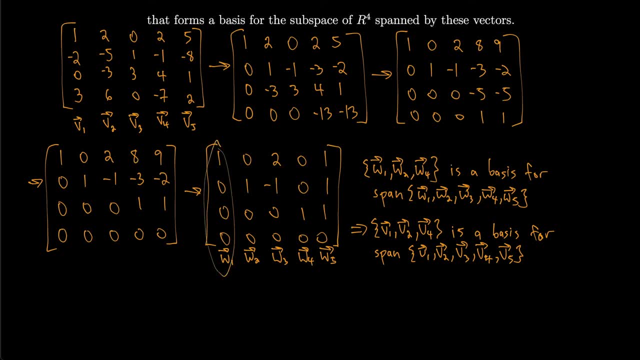 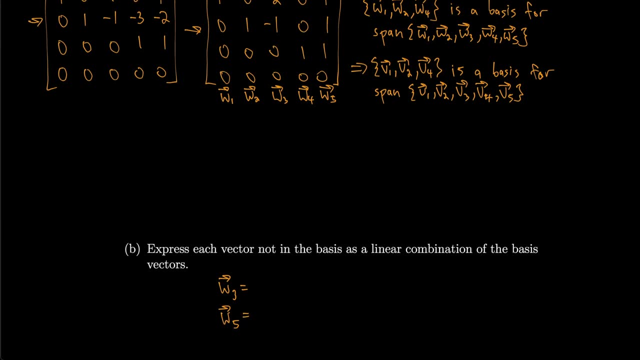 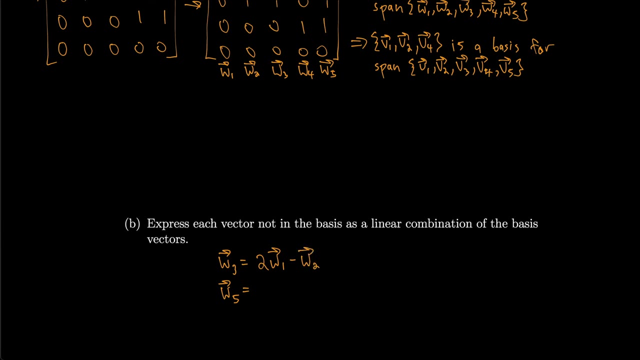 2 of W1, and we could subtract off 1 of W2, but then we get a 2 over here and a minus 1 over here, right? So it would be 2, W1 minus W2.. That's how we could build W3.. 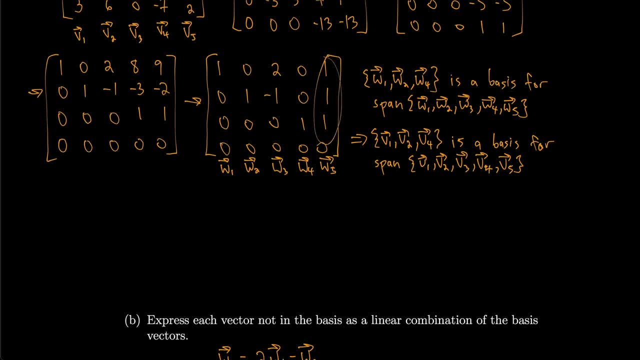 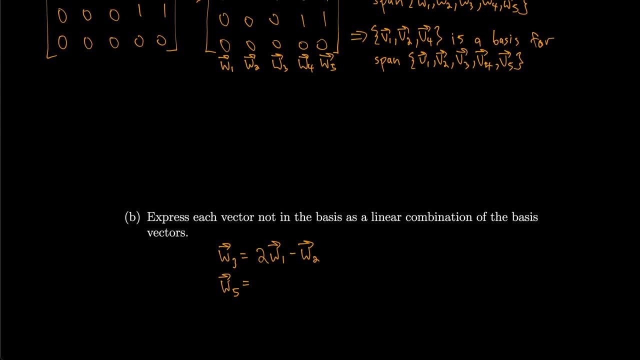 And for W5,. well, I just have 1,, 1,, 1,, so I guess we could just take this one plus this one, plus this one, 1,, 2, and 4.. So let's do that. 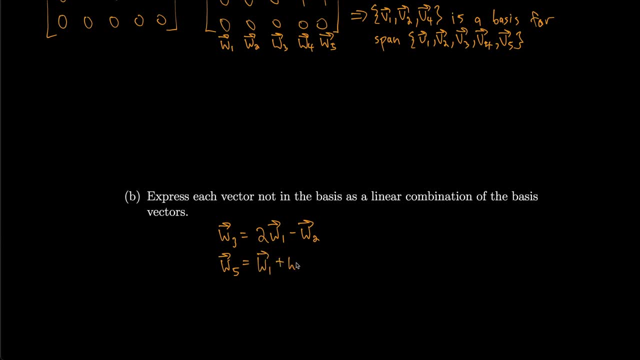 Take W1 plus W2 plus W4.. Okay, but W3, we want to translate this to the original vectors. so that means that W3 should be equal to 2 times W1 minus 1 times W2, and you can check that that's actually true. 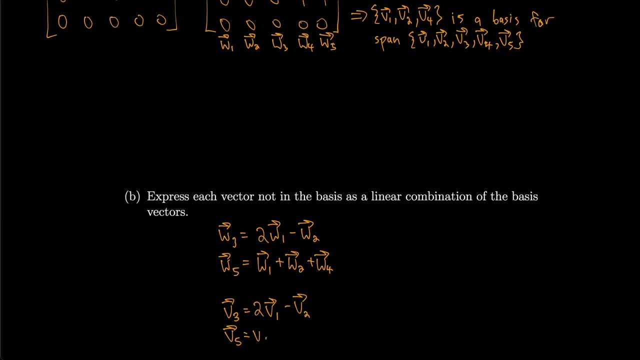 and W5 should be equal to W1 plus W2 plus W4.. And these equations, where we rewrite the vectors that are linearly dependent on the other vectors in terms of the other vectors, are called dependency equations, Should make sense because these are the linearly dependent column vectors.